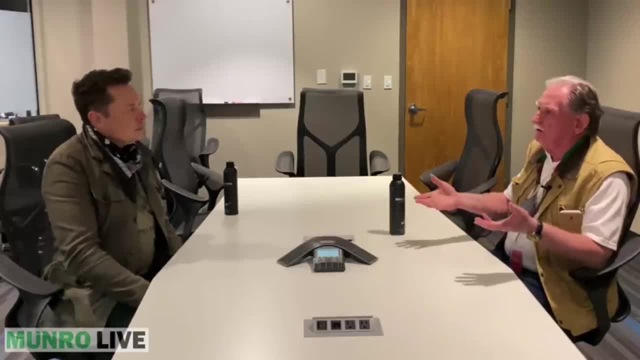 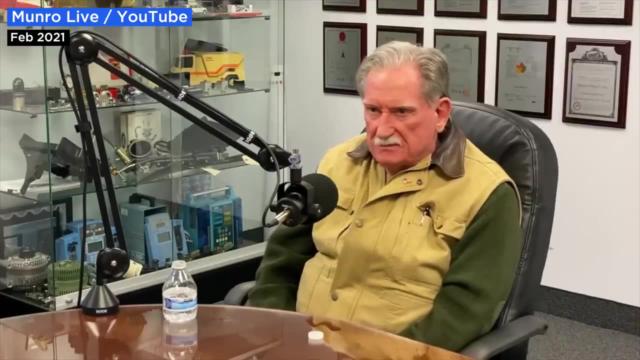 Munro Live. he said it's Musk's knowledge that stands out. Sandy Munro, Engineering Consultant. I was blown away. I've seen dozens of CEOs. I've never seen a CEO ever, or a president, that knew more about the product. 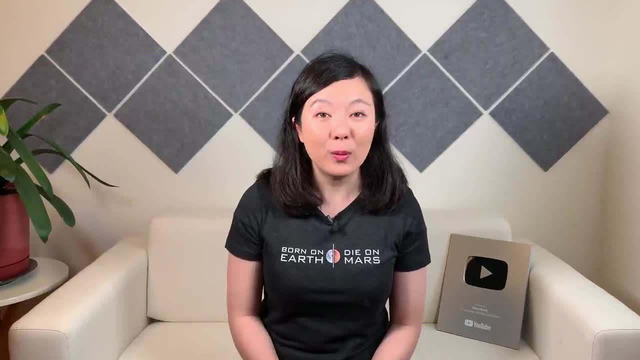 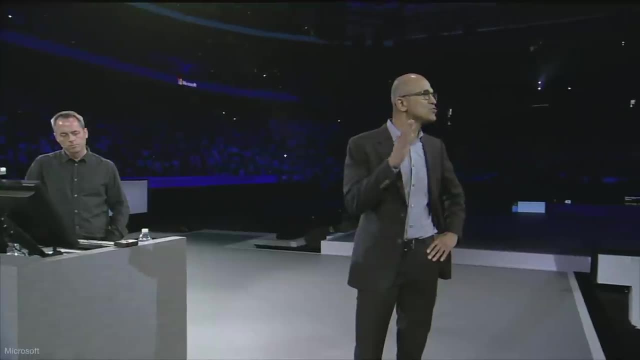 That technical know-how that comes with an engineering background goes a long way toward building better products. Just ask Satya Nadella, the engineer at Microsoft, who rose to become CEO When he took over the top job in 2014,. he had to figure out a way to make Microsoft. 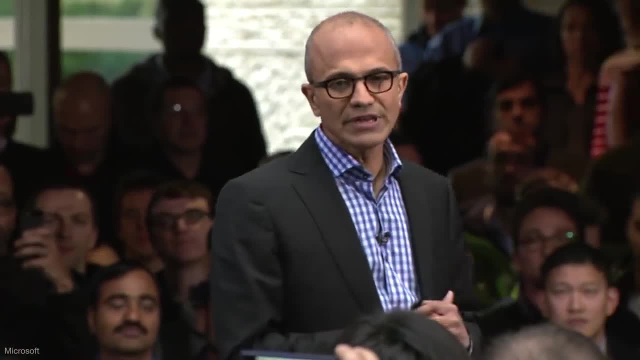 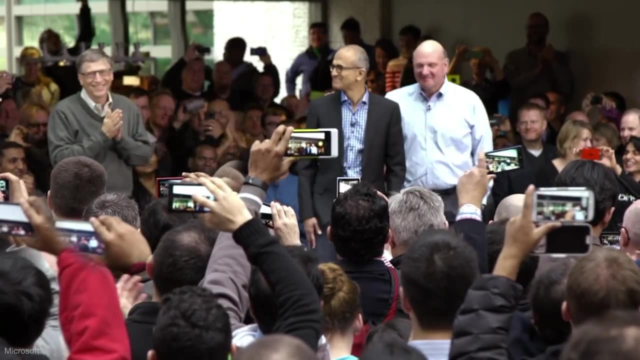 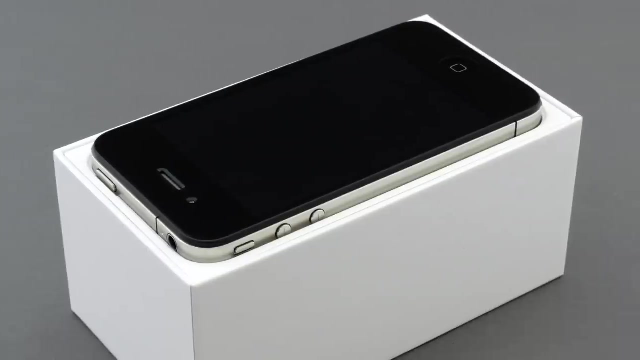 relevant as it faced an onslaught from Apple. We now need to make Microsoft thrive. The software company struggled to thrive under the leadership of his predecessor, Steve Ballmer. Its products were far from revolutionary. The Surface was a response to the iPad, the Windows phone an answer to the iPhone. Ballmer has a degree in mathematics. 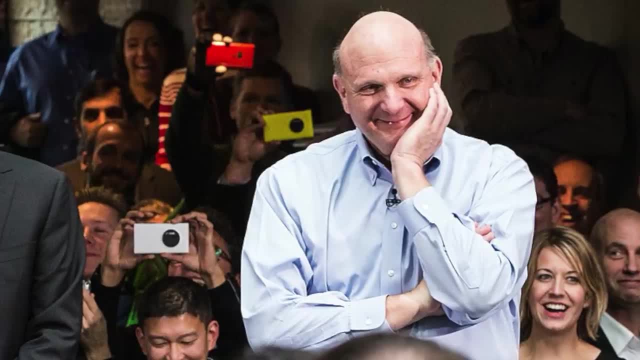 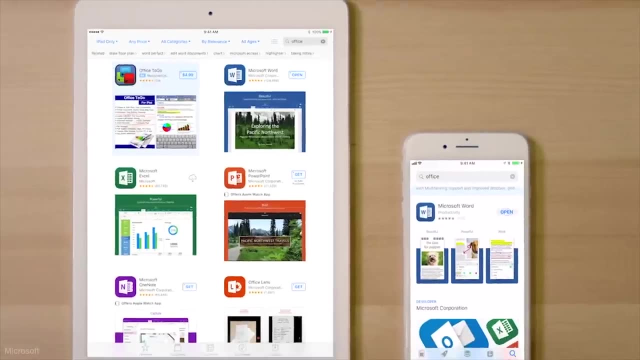 and economics from Harvard, which helped balance the books, but didn't do much when it comes to innovation. When Nadella took over, he transformed Microsoft, moving its software to non-Windows devices, For example, bringing Microsoft Word to the iPad and the iPhone. He also 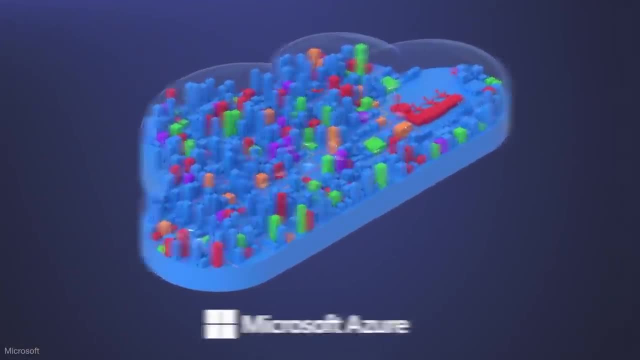 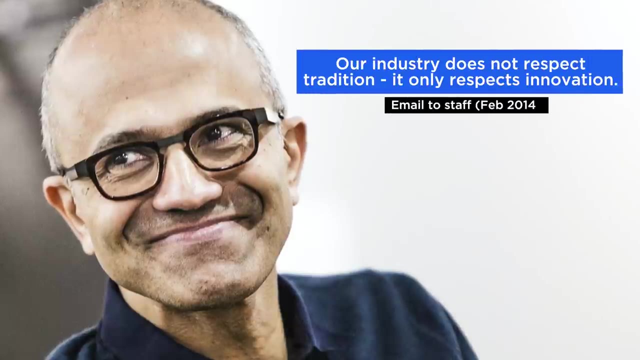 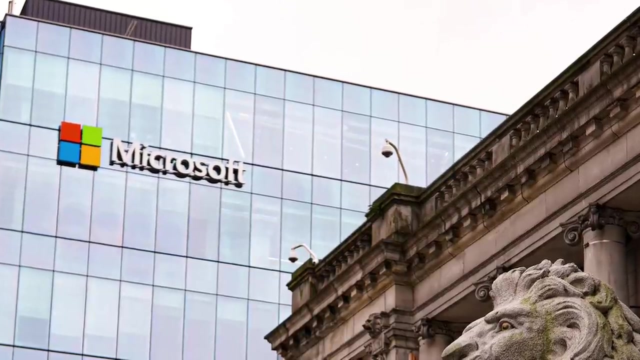 expanded its cloud business, Azure, which has become the biggest rival to Amazon's AWS. In his first email to employees, as CEO Nadella wrote, Our industry does not respect tradition. It only respects innovation. That innovative spirit of engineering saved Microsoft. 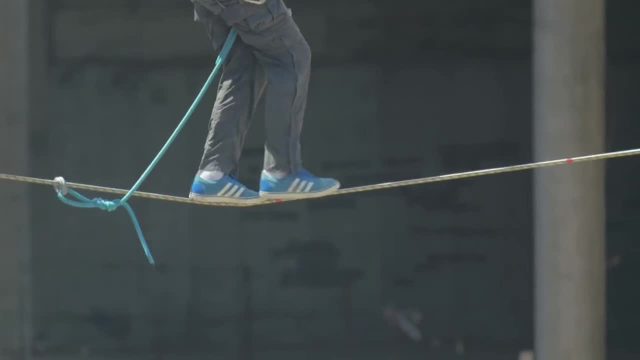 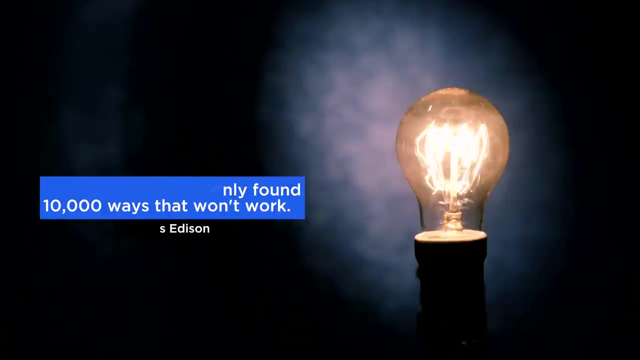 But it's not easy. It requires risky moves and not accepting failure. As American inventor Thomas Edison famously said: I have not failed, I've only found 10,000 ways that won't work. James Dyson, the British engineer, knows a thing or two about not giving up. He became frustrated when a vacuum 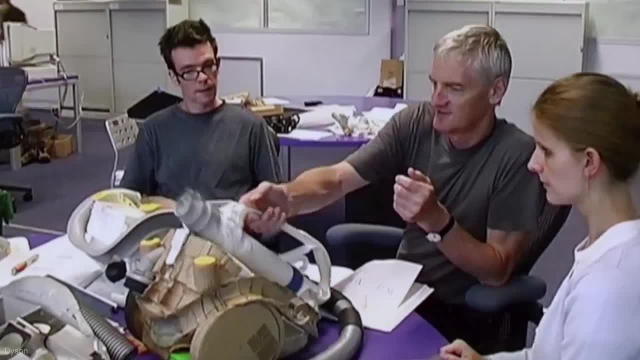 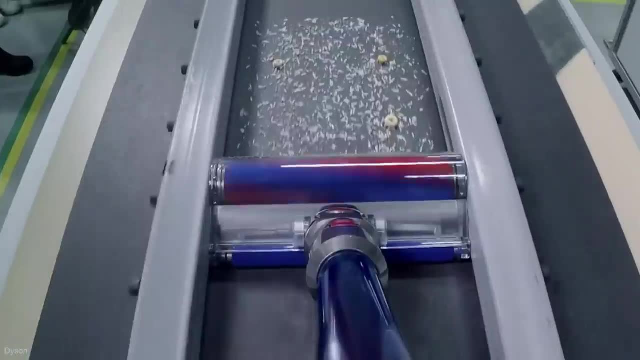 he had at home kept losing suction, so he decided to build a better vacuum himself. He spent 15 years tinkering with over 5,000 different prototypes to come up with the perfect bag-less design. I'd like to give you a little demonstration. 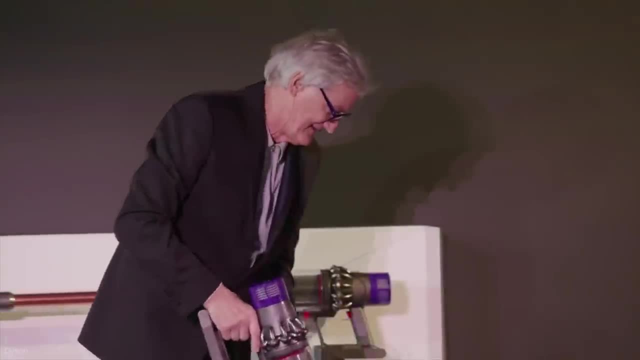 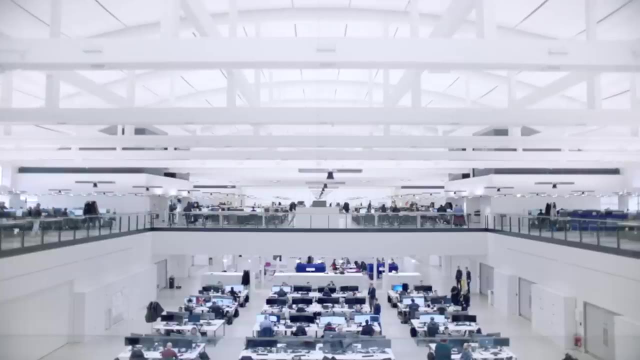 The payoff for his perseverance was a multi-billion dollar company that bears his name. In order to be successful, Dyson was invested in the fine details of his company. Engineers aren't afraid to get involved in the day-to-day business, especially when it comes to hiring.